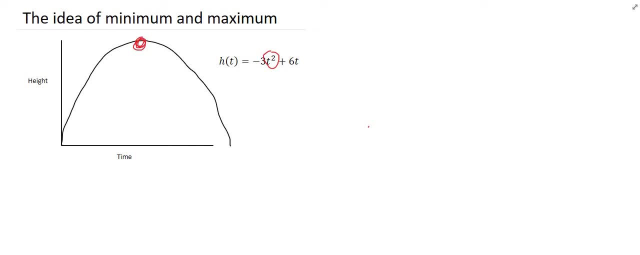 be using y and x, but we could use other variables, But the process is always going to be the same. Let's have a look. So here's our first practice question. They tell us that the side lengths of a rectangle is depicted in the diagram below, So we can see that one of the lengths is x minus 7,. 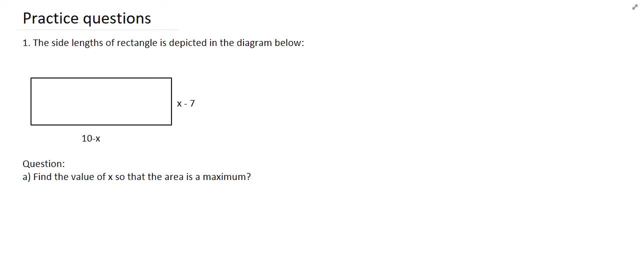 and the other one is 10 minus x Question: find the value of x so that the area is a maximum. So, straight away, what are they wanting us to? find The maximum of area. So we go, develop an equation for area. Now we know that the area of a rectangle 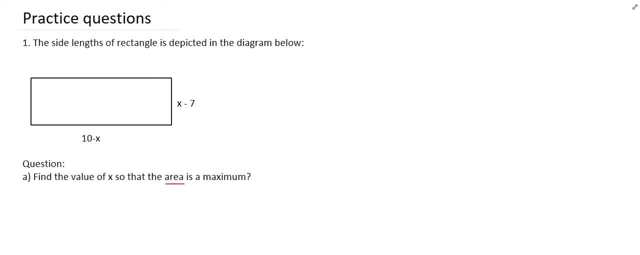 is length times breadth. So we can write that out as follows: So there we've got an equation: area is equal to length times breadth. So I've just put the length and the breadth next to each other, as if you are multiplying, And then we could go multiply those brackets together. 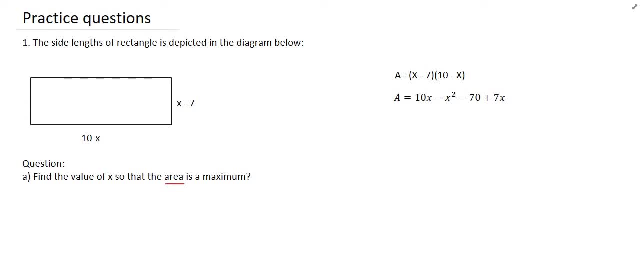 And then we could simplify all the like terms, And there we can see a parabola type of equation once again, where a is normally, your y is normally represented with the letter y, And then on the right we still have x as per normal. The point is: is that this? 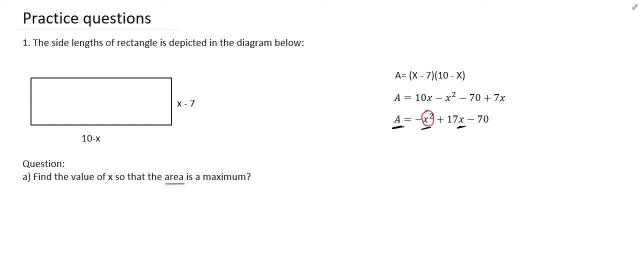 is a parabola. A parabola, remember, has the x2.. And so all that we need to do to find minimums or maximums. if you visualize a parabola, it's always going to be at the turning point, So we just find. 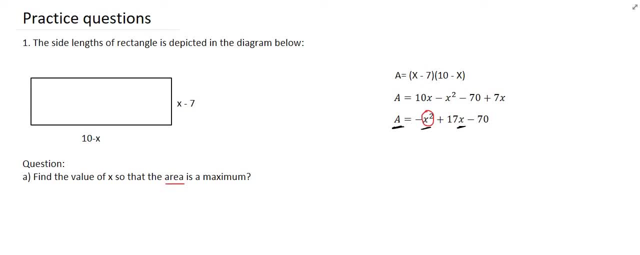 the turning point of this equation By using the equation of minus b over 2a And if you have to go, and if you have to go and sub in the b value and the a value, you're going to get an x answer of 8,5.. Please remember that that is. 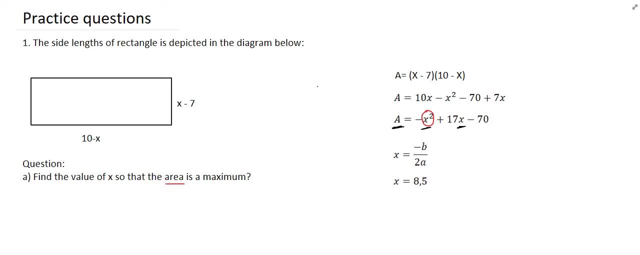 the value of x. If the question wants you to work out what the area is, well then you simply have to go plug in the value of x in the area equation which we had written over there, or you could even use that, or you could even use that one over there. But 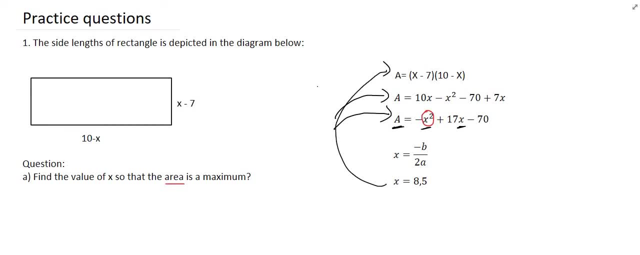 luckily for this question, they only asked us to find the value of x. they haven't asked us to find the area. If they did, we would simply have to do one more step. Let's go to another example. Here we have the height of a ball. They tell us that the height of a ball as a function of time. 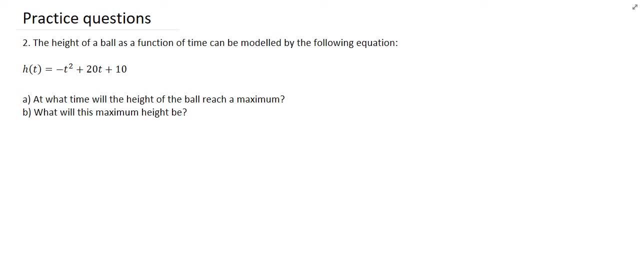 can be modeled by the following equation: And then they've given us the equation as h of t, that normally that says f of x or something like that. It just tells us that it's the y axis is h and the function uses t on the x axis. First question says: at what time will the height of the 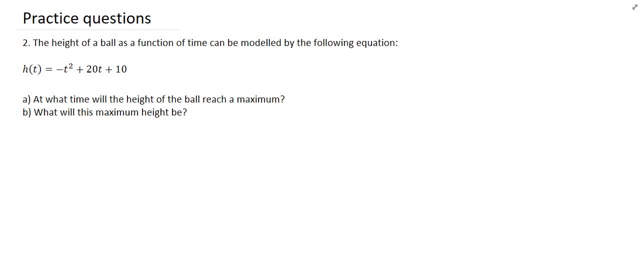 ball reach a maximum. So, remember, this is a parabola And, specifically, the fact that this is a minus means that it is a sad parabola, which means that it does reach a maximum, right, Because it looks something. 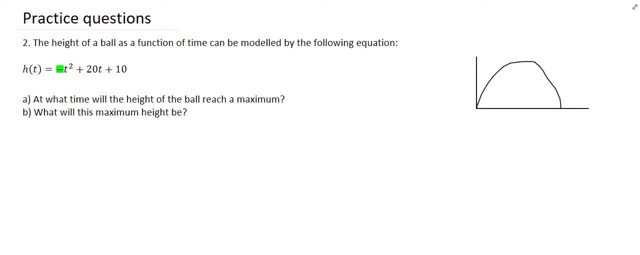 like that. Notice I haven't got a negative y axis and a negative x axis, because when you are busy with height of a ball and time those don't become negative. So to find the maximum height of the ball we simply have to find the turning point. So we can just use minus b over 2a for that equation. 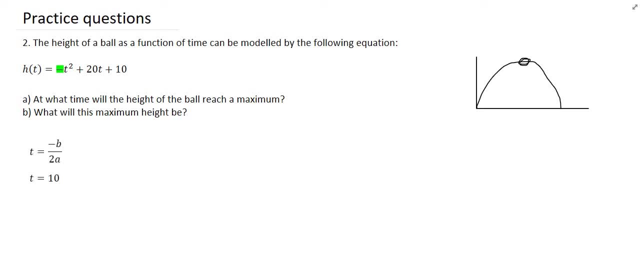 And if you do that, you're going to get an answer of: we got a value of 10.. Notice, in the formula, we're not saying x is equal to, we're saying t, because in this case our x axis is not called x anymore, it's called t. That doesn't matter, though, because it's still. 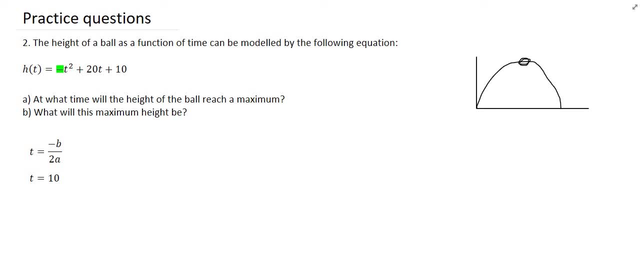 a parabola. So that's a's answer. At what time? 10 seconds. What is that height? Then you simply substitute 10 into the original equation. Notice that wherever there was a t, we have replaced it with 10.. We didn't replace that minus stays on the outside, or sorry, this minus here stays on. 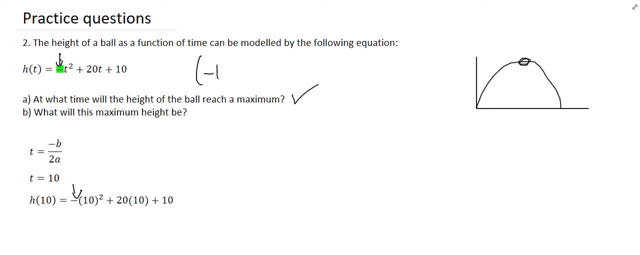 the outside, because it wasn't minus t squared, That was a negative y. So we're going to get a result that would have been like this: It was only the t that is squared, And if you had to go calculate all of this, you're going to get an answer of 110.. And then we don't really have units. 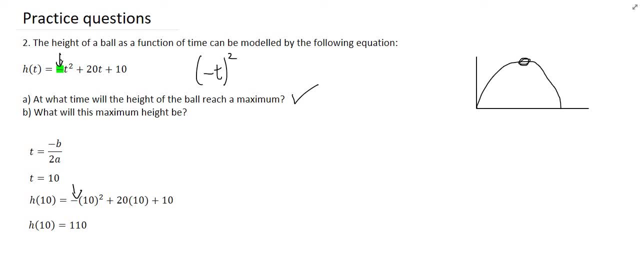 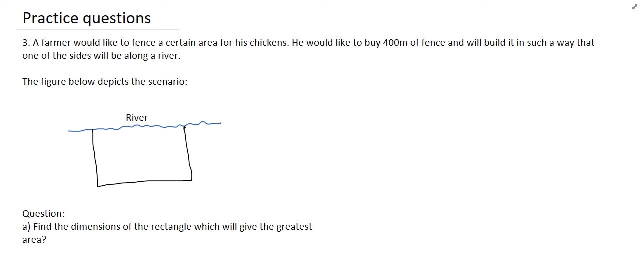 but usually in an exam they would have given units. So let's say 110 meters And that will be the height of the ball at 10 seconds. Let's try another example. The last question for this video tells us that a farmer would like to fence a certain area for his chickens. 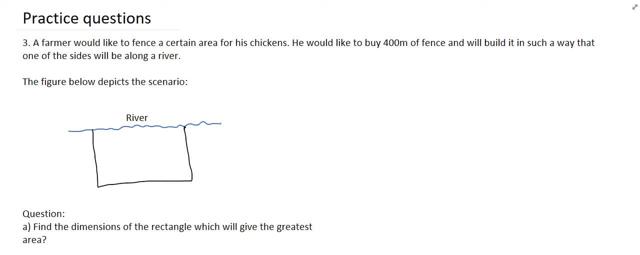 he would like to buy 400 meters of fence and will build it in such a way that one of the sides will be along a river. the figure below depicts the scenario. find the dimensions of the rectangle which will give the greatest area. so we want it to be a maximum. so what we could do, for example, 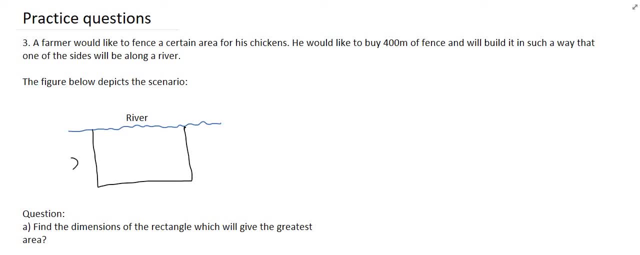 is. we could call this side here. we could call that x, then because of a rectangle, this will also be x. you could then call this one y, but now we have too many variables. we've got x and y, but luckily we know that this man can only buy 400 meters of fence, so we know that this. 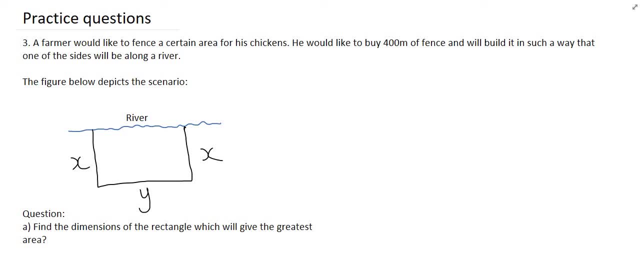 these all three sides should add up to 400, so we can make a formula as follows: then we could simplify the 2x, the x and the x and make that 2x, and then we could get y by itself. now they asking us to find the, the, the dimension, so that the area is a maximum. so we need to create a. 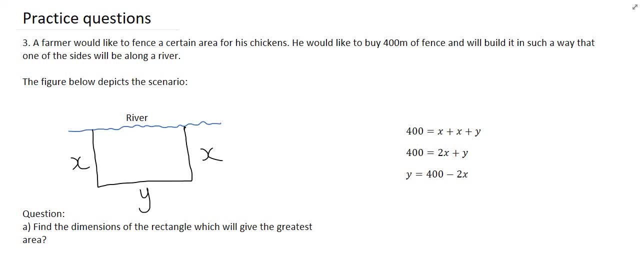 formula with area. so we know that area of a rectangle is equal to length times breadth. so let's do that. and then for that area equation we can't have x and y, but luckily we know that y is the same as 400 minus 2x, and so we can replace it in the place of y. then we could multiply that. 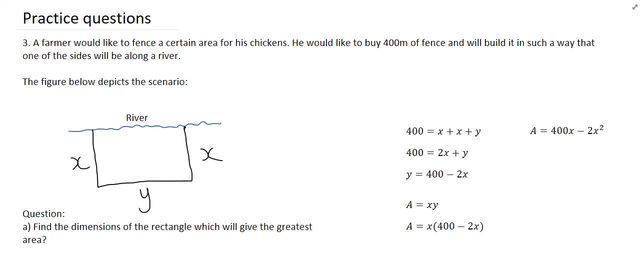 equation. now we could first rearrange that equation so that the x squared is in the front, and then we could use minus b over 2a to get the x value of the turning point. and so x is 100. then the question asks us to find the dimensions. so we know what x is. it's 100, which means that. 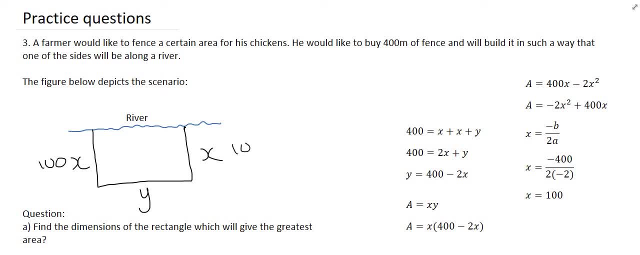 this is 100, this is 100. and then we also know from this equation that y is equal to 400 minus 2x, and so if you had to plug x into there, you'd get a y answer of 200. notice that the question doesn't ask us to find the maximum area, so we can stop right there. if they did ask us to find. 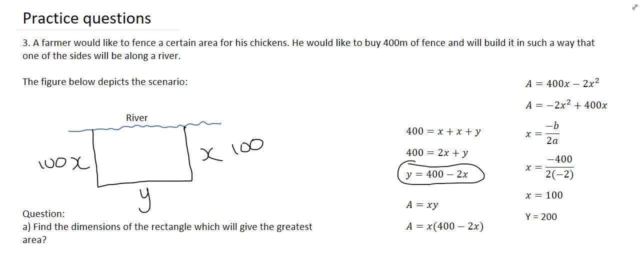 the maximum area, then you would just plug your values into the equation for the area and get your answer, and that is the end of this video.